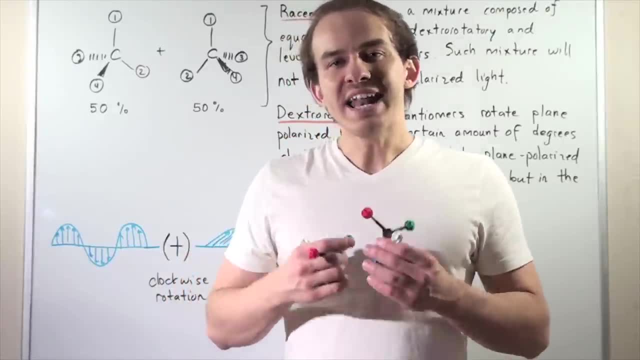 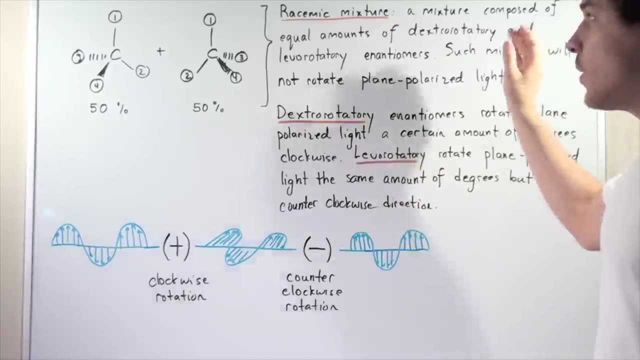 in the counterclockwise direction. So what happens if I create a racemic mixture? Now, a racemic mixture is a mixture composed of equal amounts of the same enantiomer. Now say if this enantiomer is cookinglı and it responds with the same erantic recommendation. 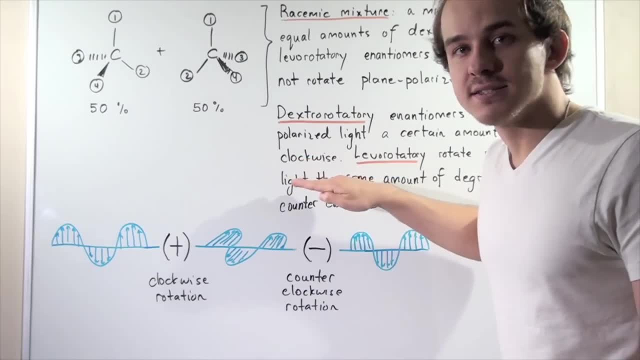 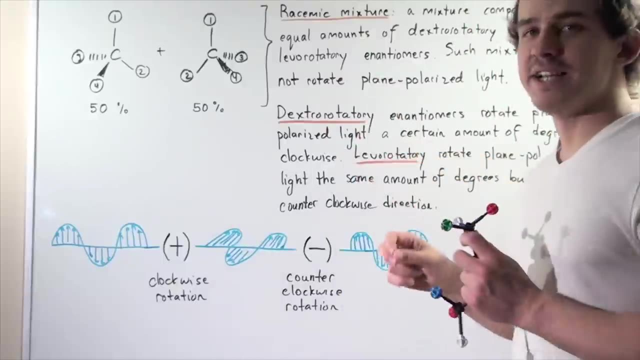 and it's continuous rotation taking the same". So just imagine an enantiomer is cooking dish and its sat nav will be stirring the flames in the center, focusing on a particular or abuse in a specific, specific way. The weaker the enantiomer, the stronger the flame. 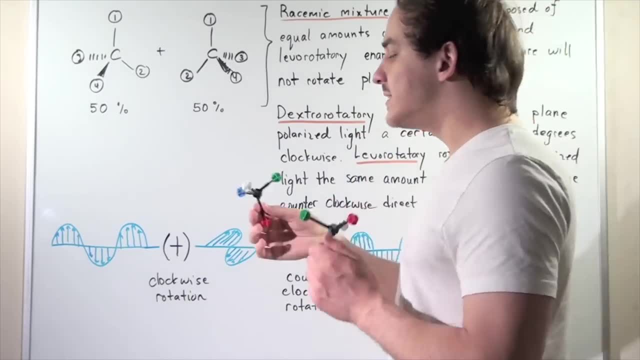 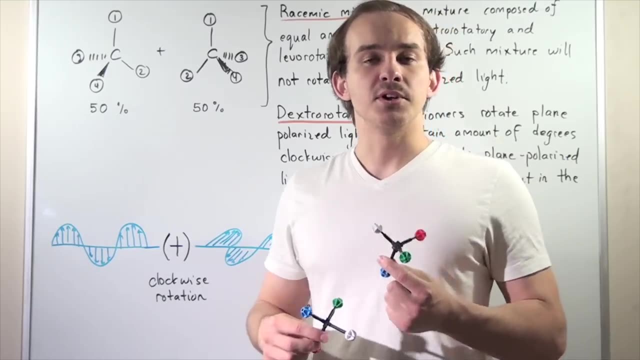 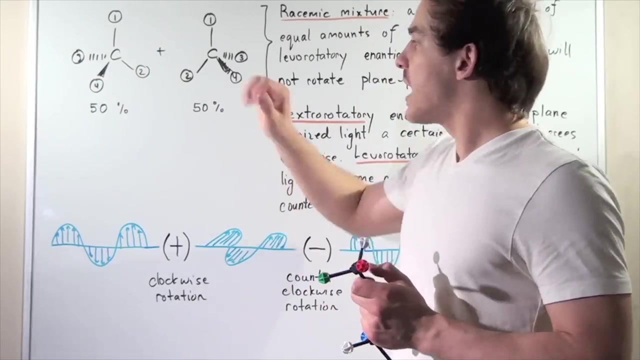 The flames will be dense and the hemical will be brighter. So what happens then is that if this silky mixture is being cooked to a tight gel, the. So in container A I have one type of enantiomer, in container B I have a second type of enantiomer, and in container C I create a racemic mixture of 50% of one enantiomer and 50% of the second enantiomer. 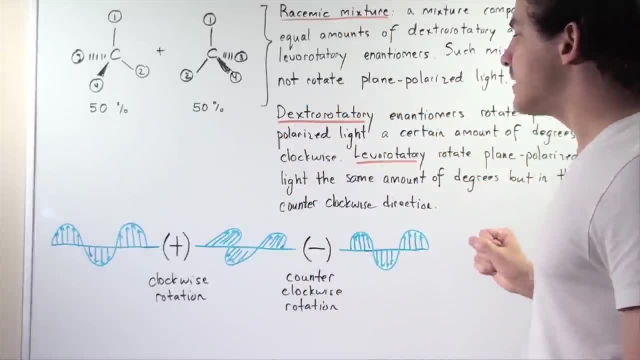 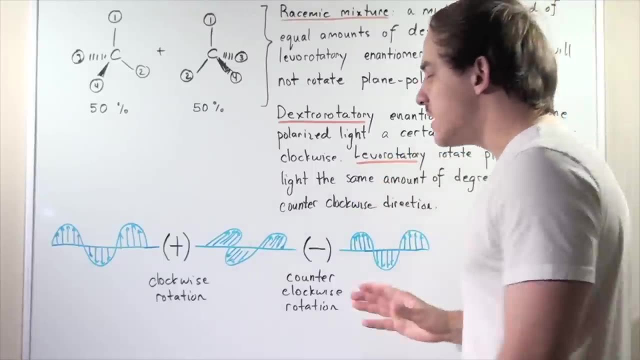 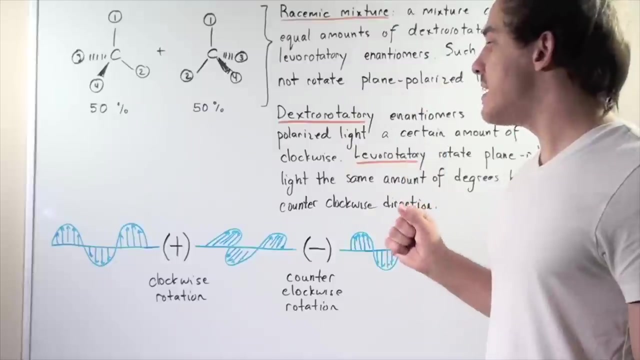 Recall that dextrorotatory is also represented by a positive sign and levorotatory is also represented by a negative sign. So let's suppose I have my mixture and I shine my plane polarized light onto my racemic mixture. 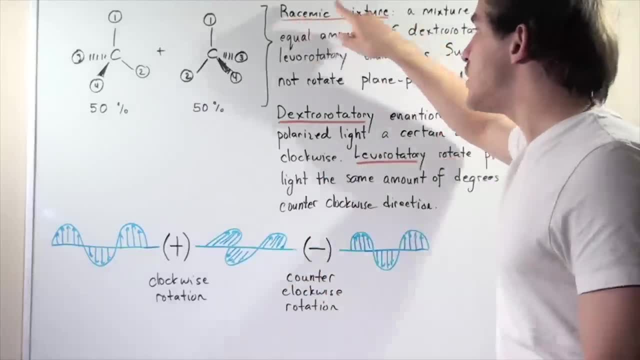 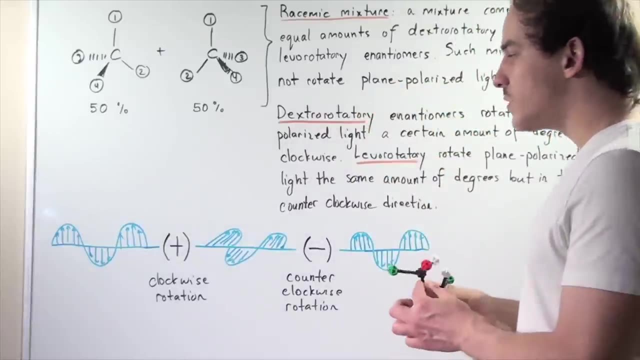 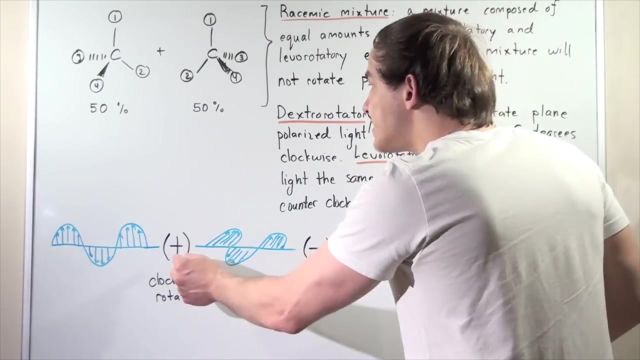 What will happen? Well, it turns out that such a mixture does not rotate plane polarized light. and let's see why that's the case. So when I shine my plane polarized light, one of the enantiomers, the positive or dextrorotatory enantiomer, rotates. 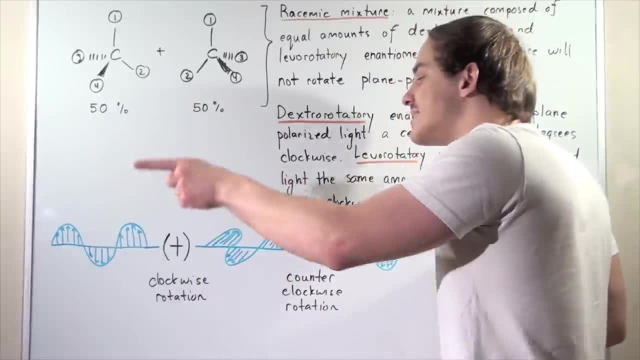 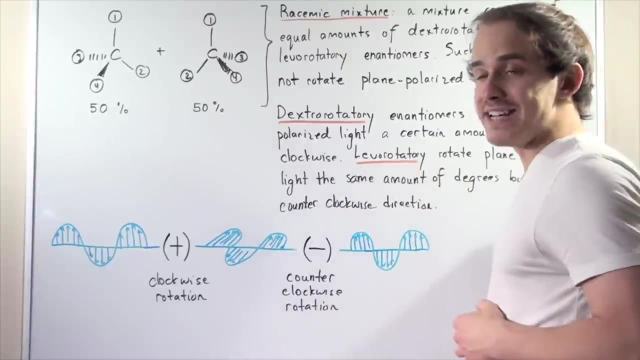 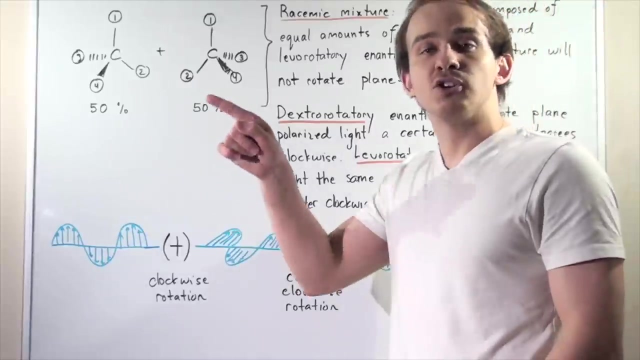 It rotates a certain amount of degrees in the clockwise direction. and then when that rotated light hits my levorotatory enantiomer, this guy undoes this rotation because it rotates it the same amount of degrees but in the counterclockwise direction. 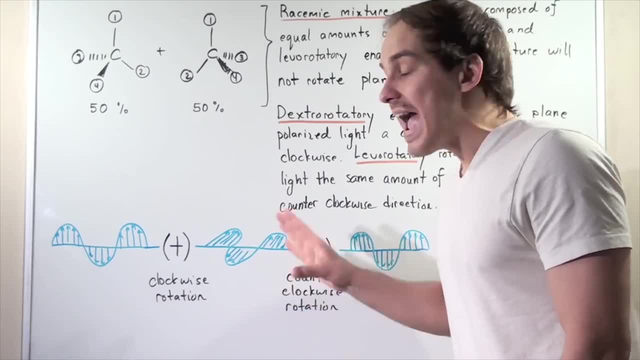 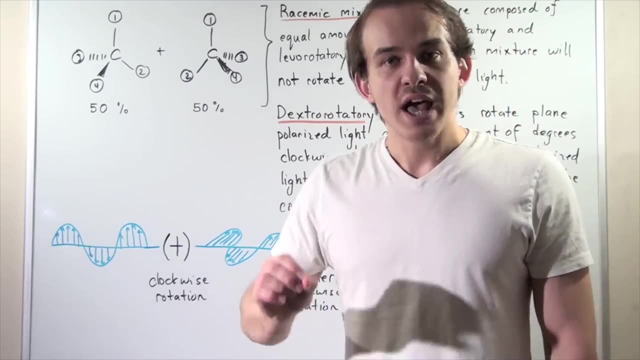 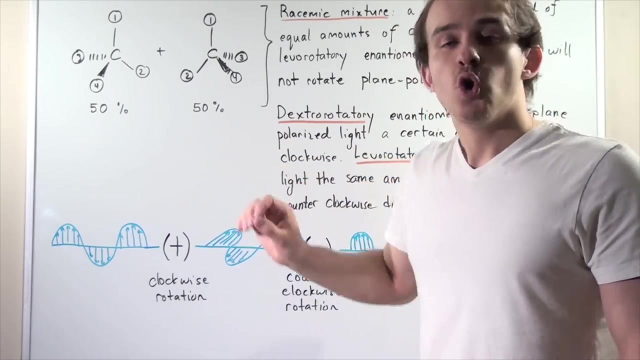 So this ray of light ends up being on the same plane as the original. So there's a net rotation, There's a rotation of zero, and all racemic mixtures- 50% of one enantiomer and 50% of the second enantiomer- will not rotate plane polarized light.